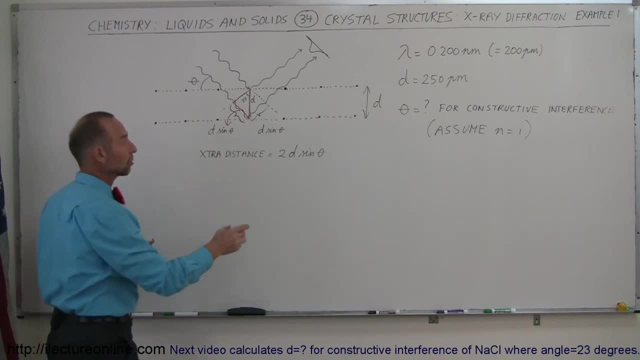 And if we set that distance equal to 1 wavelength, we can actually solve that equation for theta. In other words, what angle do we need to? does the beam have to approach the crystalline structure in order to get constructive interference? So 2 d sine theta is going to be equal to 1 wavelength. 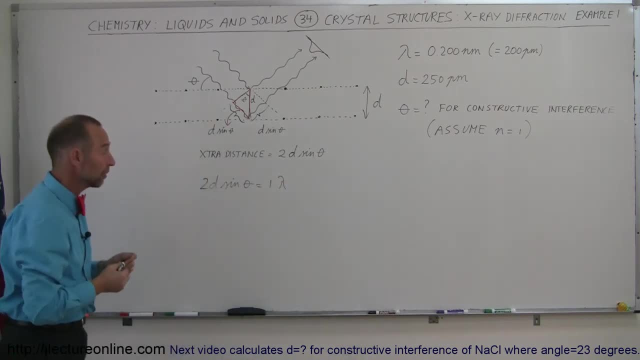 At that point we will see constructive interference. Of course, if it's equal to 2 wavelengths or 3 wavelengths, again we'll see constructive interference. But we may not have achieved that because there may be limitations as to how many times we can get constructive interference as we change the angle. 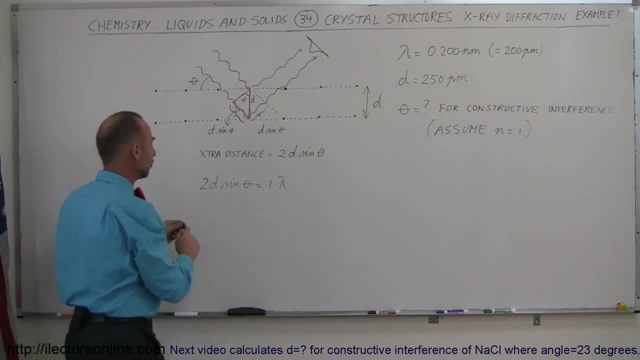 And you'll see that in just a moment. So let's solve for this angle first. So now we have: the sine of theta is equal to the wavelength lambda divided by 2 times the separation distance, And so therefore theta is equal to the arc sine of lambda divided by 2.. 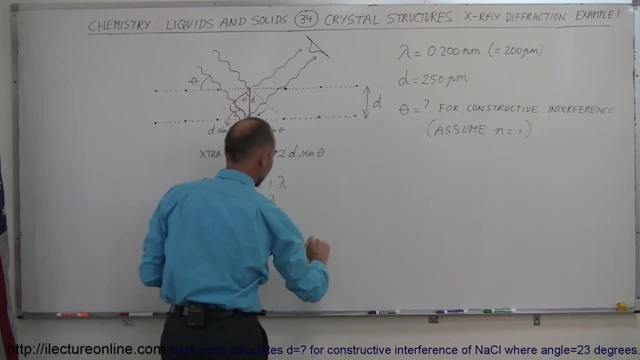 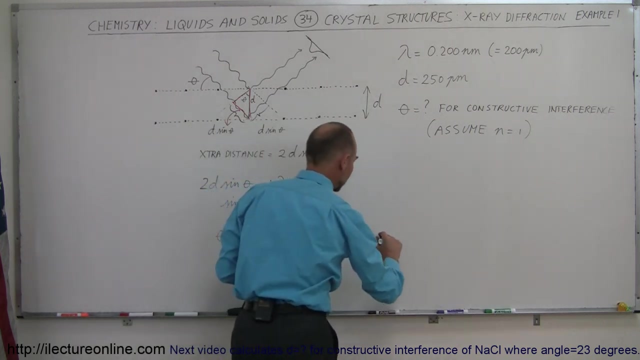 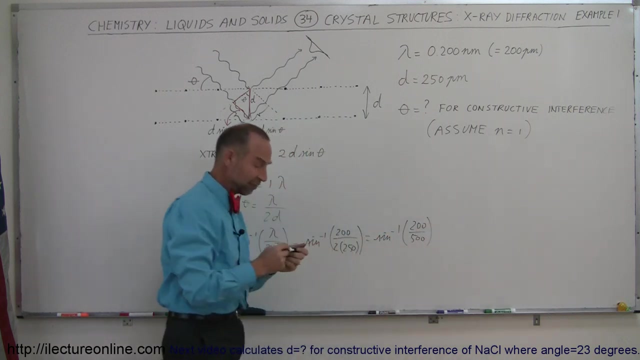 2 times the separation distance, which is equal to the arc sine of lambda, which is 200 picometers divided by 2 times the separation distance of 250 picometers. So that would be the arc sine of 200 divided by 500, which is the arc sine of 0.4.. 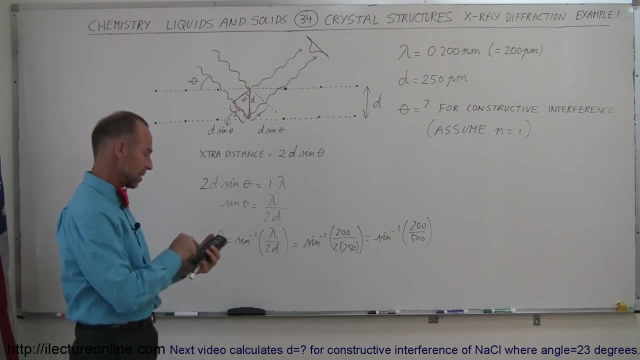 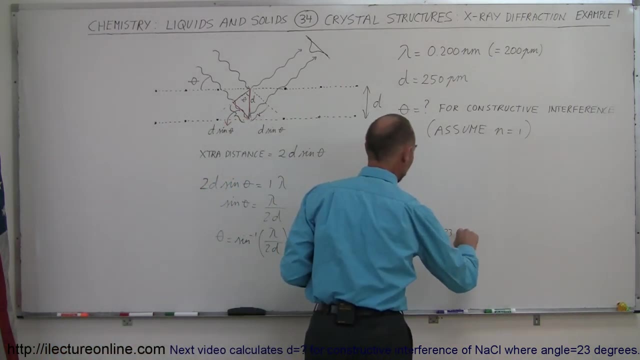 And with a calculator we'll find out in just a moment what that is: 0.4.. And we'll find out what that arc sine is And we get 23.6 degrees. So that's equal to 23.6 degrees. 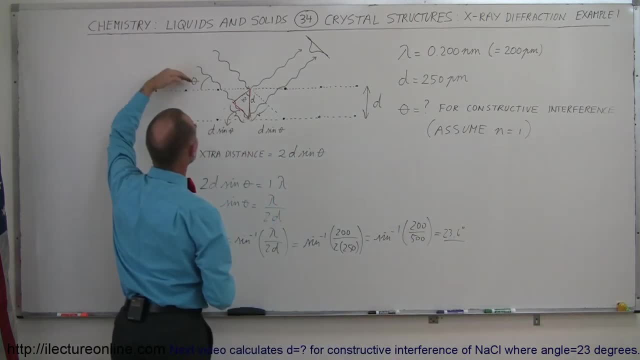 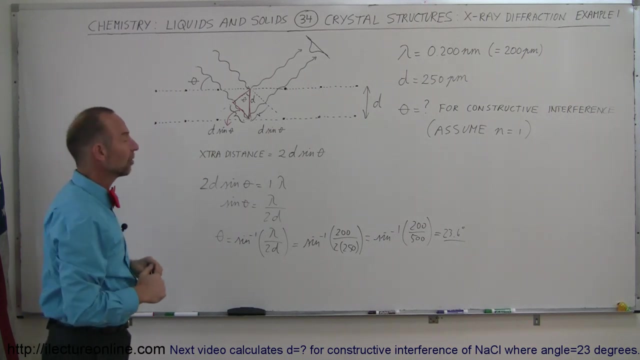 So if we angle the beam in such a way that the beam is angled in relative to the horizontal at 23.6 degrees, we'll get constructive interference. The detector will see both beams being in phase, say OK. From that we can then surmise what the separation distance is. 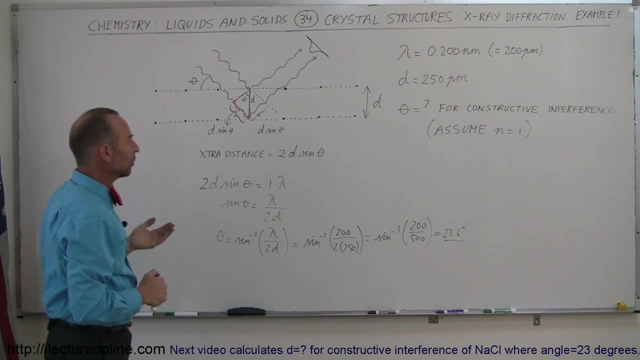 Notice that we could probably increase the angle and find a way to get the constructive interference when the wavelength difference is 2 lambda. So let's try that, Let's see. let me use a different color here. let me use green. So what we're going to do now is we're going to do the same equation. 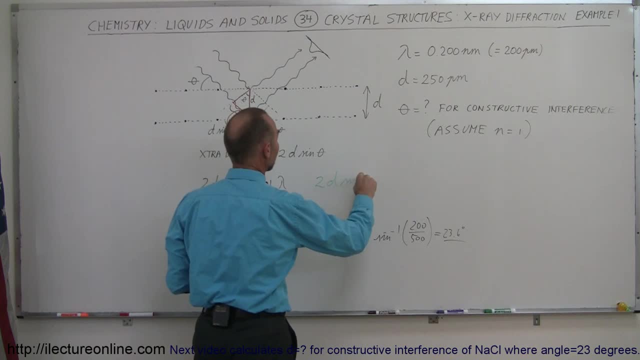 but now we're going to set the extra distance, 2d sine theta. We're going to set equal to 2 lambda and see if we can find an angle as a solution there as well. So first of all the 2s cancel out and so we have the sine of theta is equal to lambda divided by d. 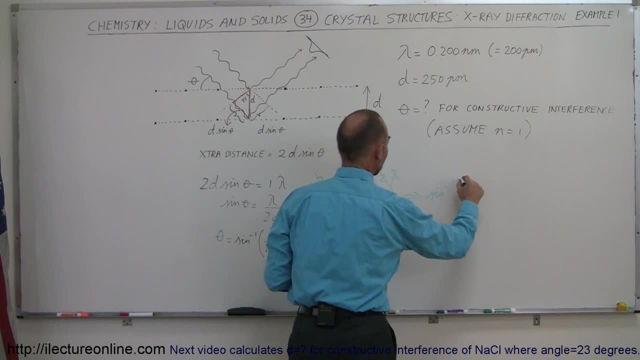 which means that the arcsine- just like before we take the arcsine- of lambda over d, the lambda would be 200 picometers and d would be 250 picometers, and that would be equal, of course, to theta. 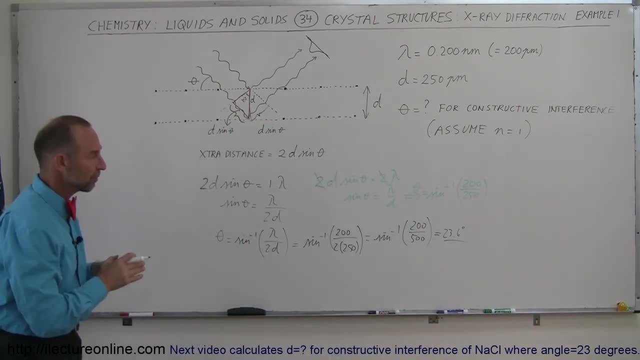 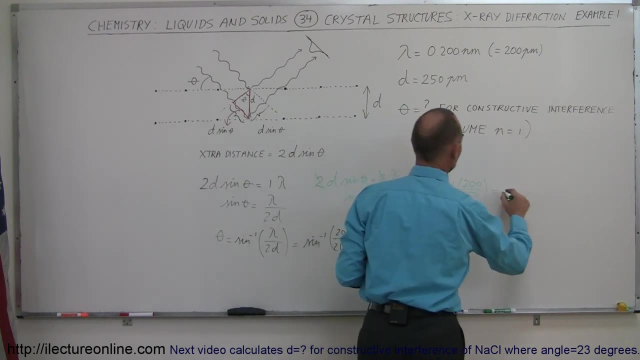 So that's a new angle. We should see another constructive interference pattern when the separation distance is equal to 2 lambda, and so that would be the arcsine of 0.8.. So let's see, Let's see what that angle is at 0.8.. 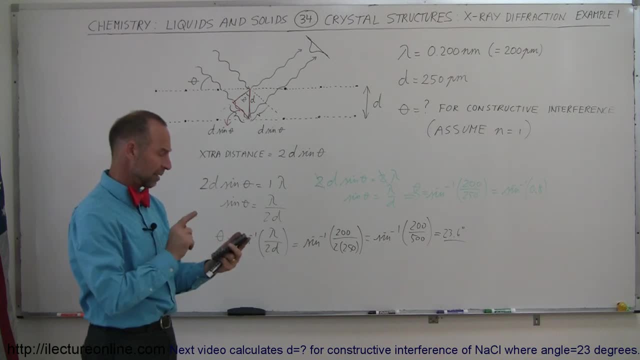 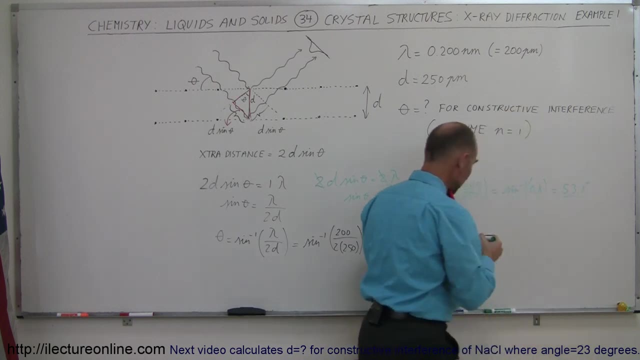 So 0.8,. take the arcsine of that and we get 53.1 degrees. so we can angle the x-ray beam at an angle of 53.1 degrees and again we will see a constructive interference pattern on the detector. 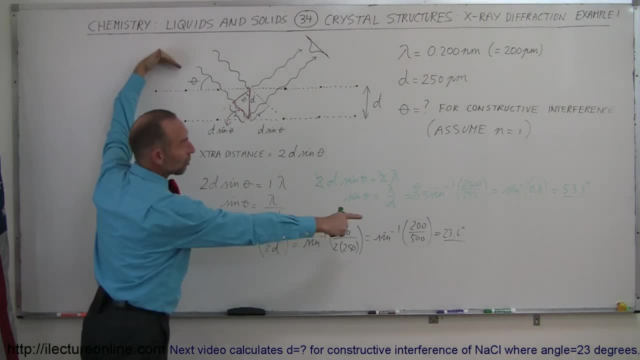 So we can start angling the x-ray beam. when we reach 23.6 degrees the detector will see a strong interference pattern with a constructive interference pattern. so we'll see a strong signal. Then we can continue to increase the angle. then what happens is the beam strength will disappear. 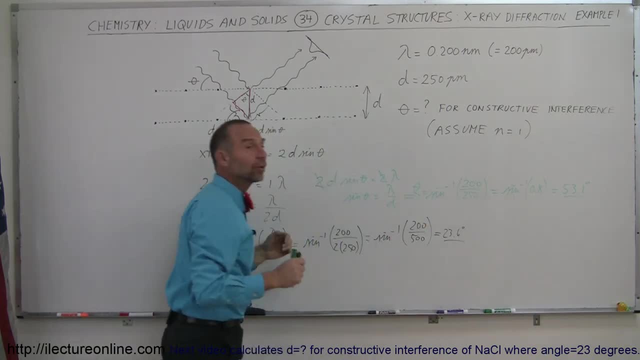 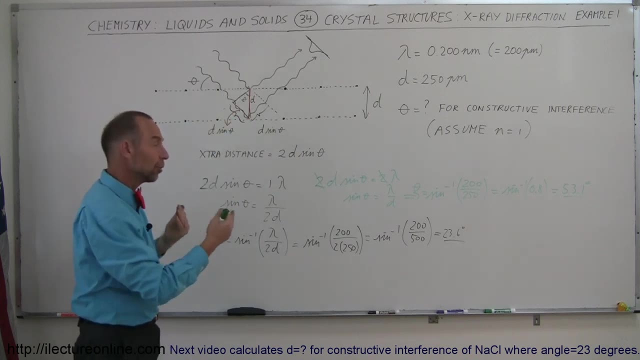 and then when we continue to increase the angle until we reach 53.1 degrees again, the interference pattern now will be strong. we construct interference and the detector will see a strong signal again. And so you can verify then that at various angles, when you'll see constructive 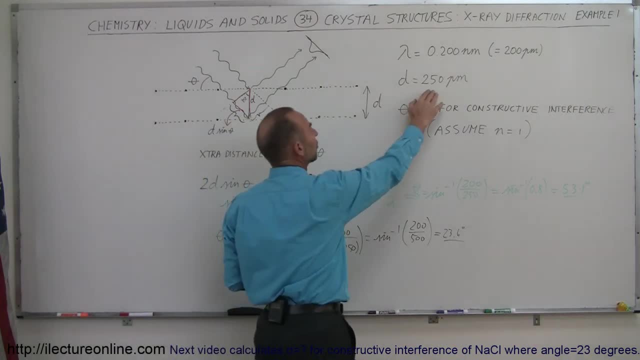 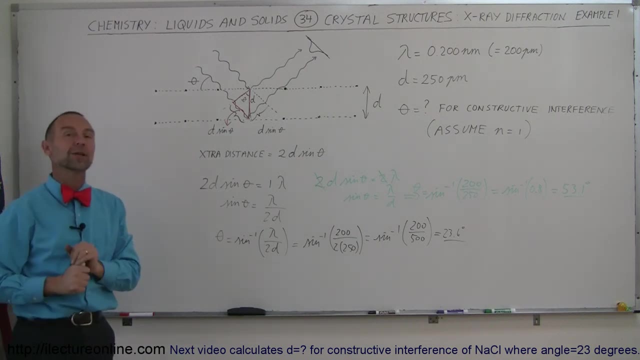 and we'll see destructive interference pattern, with a result that we can actually figure out from those angles what the separation distance is, of course knowing that the wavelength of the x-ray is 200 nanometers. So there's a nice example, and let me do one more video with an example at a slightly different slant. 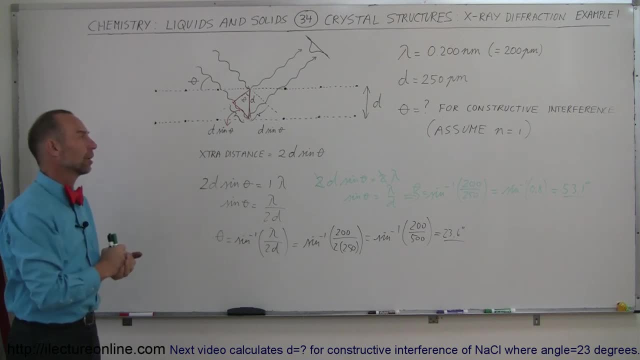 so you can feel very comfortable on how to find the separation distance between the layers in a crystal structure by using these x-ray diffraction pattern techniques.